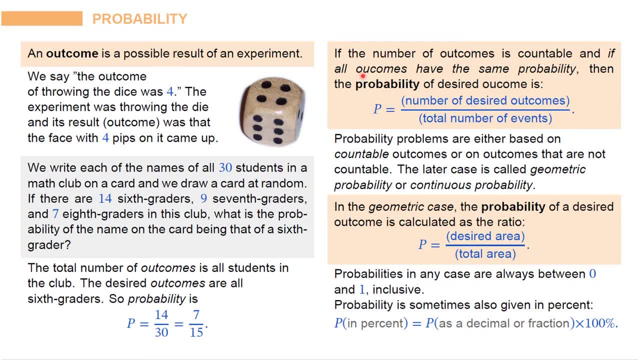 seven over 15.. If the number of outcomes can be counted and if all outcomes have the same probability, then the probability of a desired outcome- sorry for the misspelling- is: p equals the number of desired outcomes over the total number of outcomes. 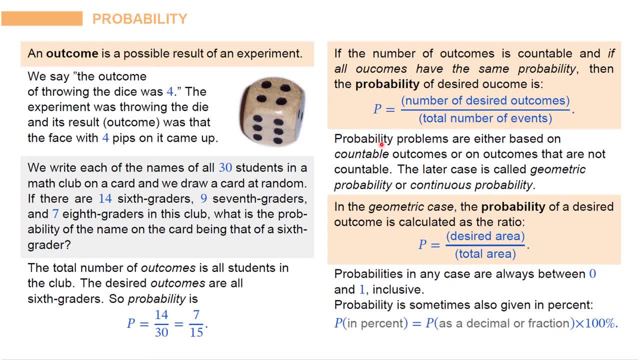 number of possible events. Probability problems are either based on countable outcomes or in outcomes that are not countable. The latter case is called geometric probability or continuous probability, and we'll actually have a lesson touching that subject later on this year. In the geometric case, the probability of a desired outcome is typically calculated as the. 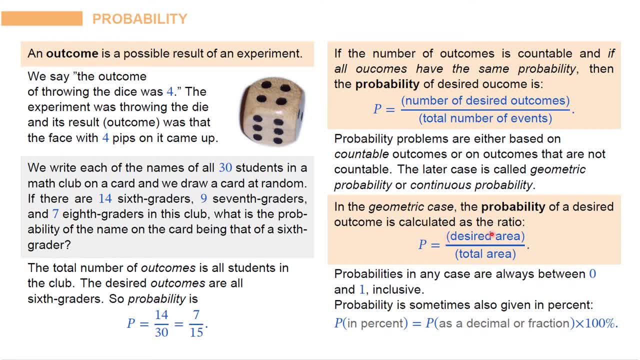 ratio p equals the desired area over the total area. In any case, whether it's countable or geometric, the probability is always between 0 and 1 inclusive. If something will never happen, the probability is 0.. If it will always happen, the probability is 1.. Probability is sometimes. 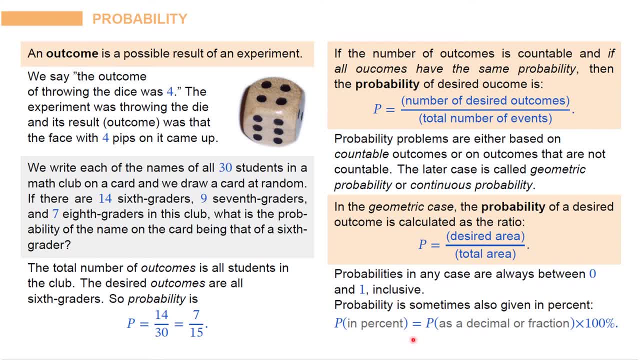 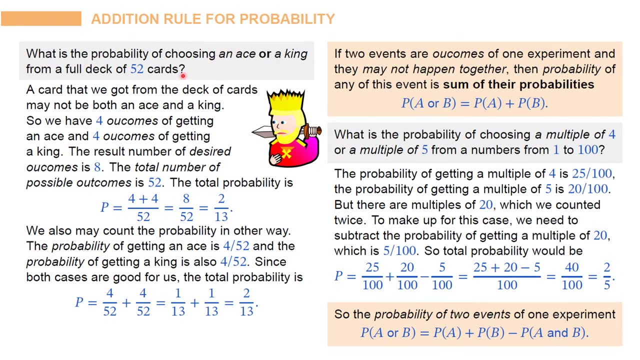 often given as a percent. P in percent is equal to the p written as a decimal or fraction multiplied by 100 percent. On this slide we're going to talk about the addition rule for probability. Let's look at the example. What is the probability of choosing an ace or a king from a full deck of 52 cards? 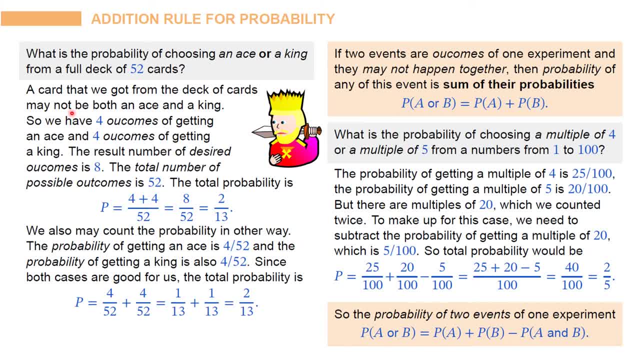 A card that we got from the deck of cards may not be both an ace and the king. We have four outcomes of choosing an ace. We have four outcomes of choosing an ace and four outcomes of choosing a king. The resulting number of desired outcomes is eight. The total number of possible outcomes: 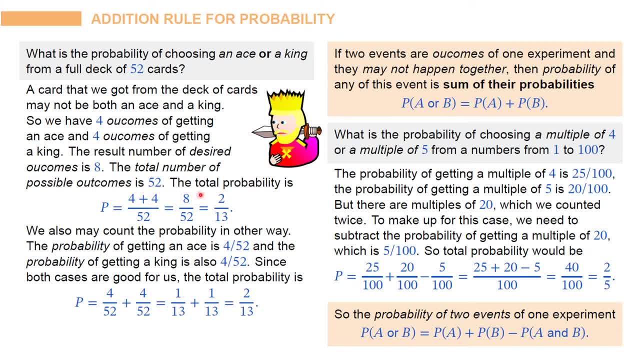 is 52. The total probability is: p equals 4 plus 4 over 52, which equals 8 over 52, which reduces to 2 over 13.. So we had these two sets of outcomes that couldn't happen simultaneously, and so we were. 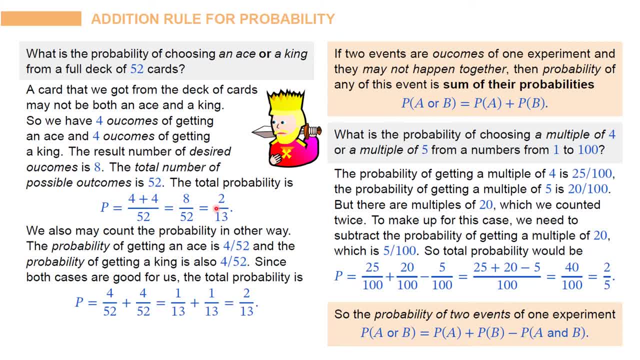 allowed to add those two outcomes together to figure out the probability of getting either outcome. So when you see, or in a problem, it's often a sign that the addition rule for probability is going to come in handy. We may also count the probability in another way: The probability of 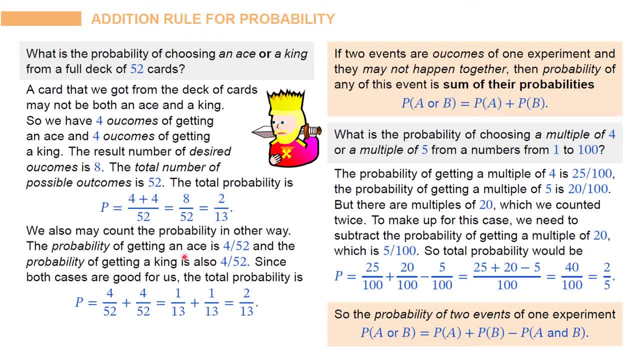 getting an ace is 4 out of 52, and the probability of getting a king is also 4 out of 52. Since both cases are good for us, the total probability is: p equals 4 over 52 plus 4 over 52,, which equals: 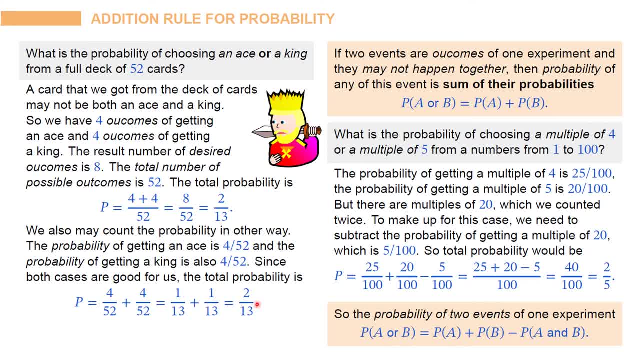 summing 1 13ths or 2 13ths. If two events are outcomes of one experiment and they may not happen simultaneously, then the probability of any of these events is the sum of their probabilities. p of outcome, A or b, is equal. 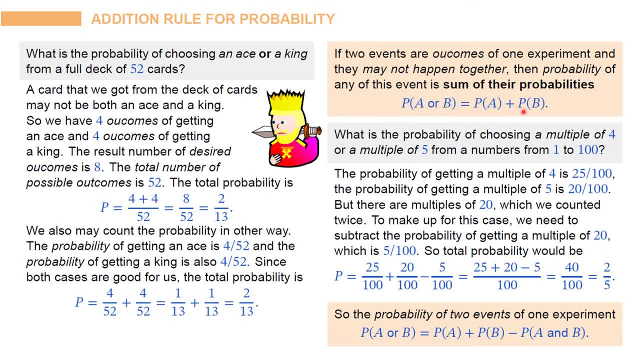 to the probability of A plus the probability of B. Now let's look at a slightly more complicated example where the probability of a is equal to b. Let's take a look at the probability of a first. The probability of a first is equal to b. Two Chili. 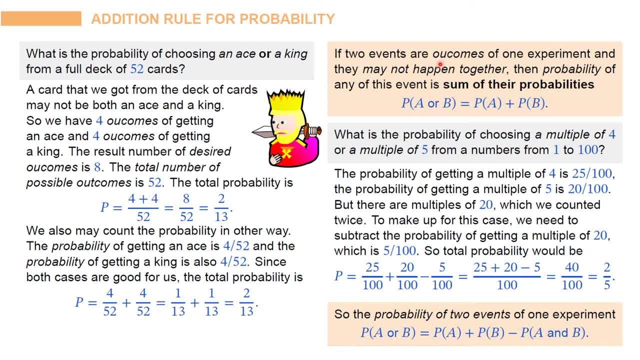 probabilities are a little bit more complicated because the events could happen together. What is the probability of choosing a multiple of 4 or a multiple of 5 from a numbers in the set of 1 to 100?? The probability of getting a multiple of 4 is 25 over 100. 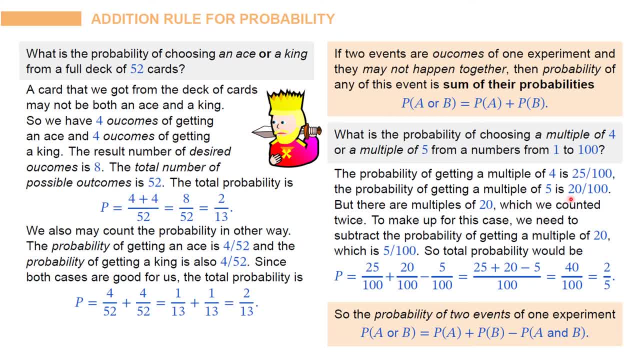 The probability of getting a multiple of 5 is 20 over 100.. But there are multiples of 20, which we counted twice. To make up for this, we need to subtract the probability of getting a multiple of 20, which is 5 over 100. 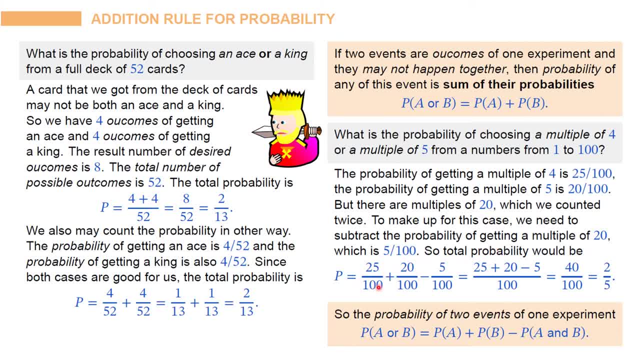 So the total probability would be 25 over 100, plus 20 over 100, minus 5 over 100, which is equal to 40 over 100, or two-fifths, So the probability of two events occurring In one experiment. 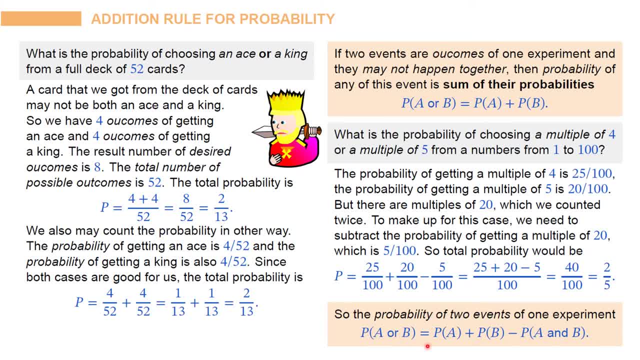 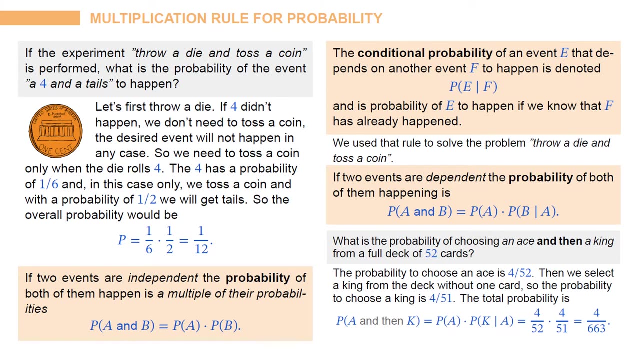 So the probability of A or B happening is the probability of A happening plus the probability of B happening, minus the probability of A and B happening. We have to subtract that to avoid over-counting. Now we move on to the multiplication rule for probability. 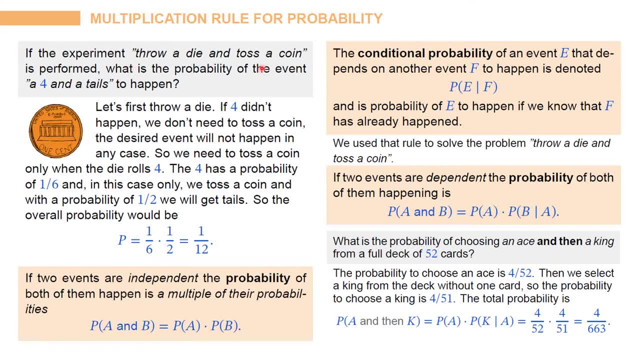 If the experiment Throw a die and toss a coin is performed, What is the probability of the event of four in a tails to happen? Let's first throw a die. If four didn't happen, we don't need to toss the coin. 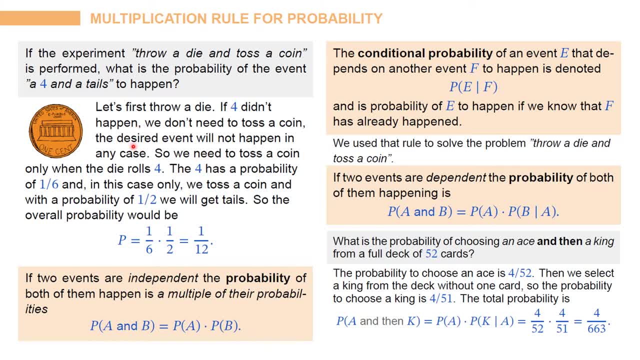 The desired event will not happen in any case. So we need to toss a coin only when the die rolls four. The four coming up has a probability of one in six, And in this case only We toss a coin and with a probability of one-half we get tails. 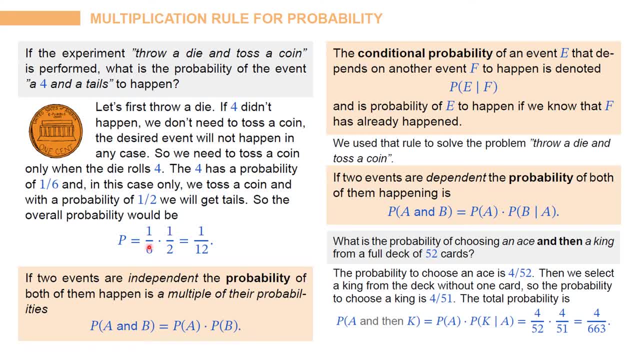 So the overall probability would be: P equals one-sixth times one-half, which equals one-twelfth. If two different events are independent, So one does not affect the other, The probability of both of them happening is a product. Okay If two events are independent. 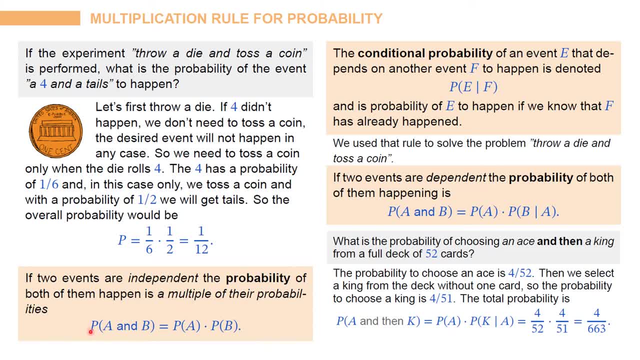 We multiply the probabilities. We multiply their probabilities together. P A and B is equal to P of A times P of B. Now let's move on to the concept of conditional probability. The conditional probability of an event E that depends on whether another event F happened. 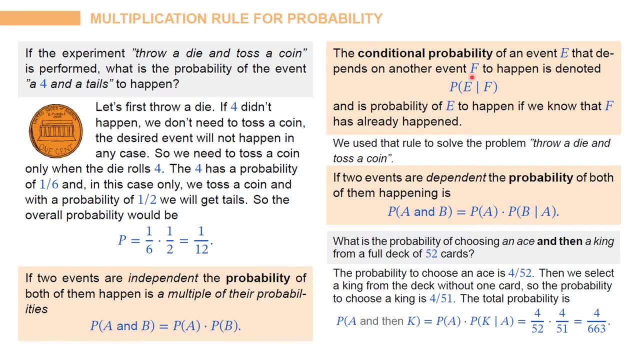 is denoted by P of E times P of B. So the conditional probability of an event E that depends on whether another event F happened is denoted by P of E times P of B. vertical line F and this is the probability of event E happening if we know that F has already. 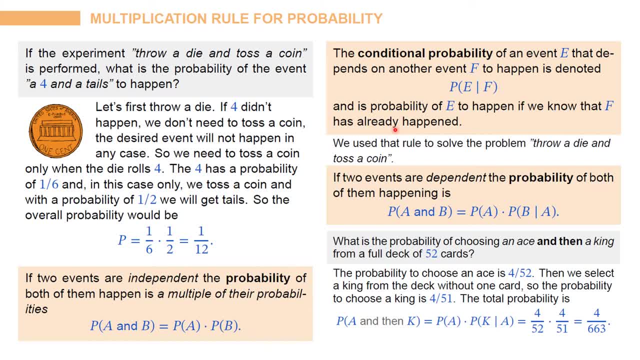 happened. We could have used that to solve the problem. throw a die and toss a coin. If two events are dependent- in other words, the second event depends on whether or not how the first one turns out- the probability of both of them happening is P of A and B equals. 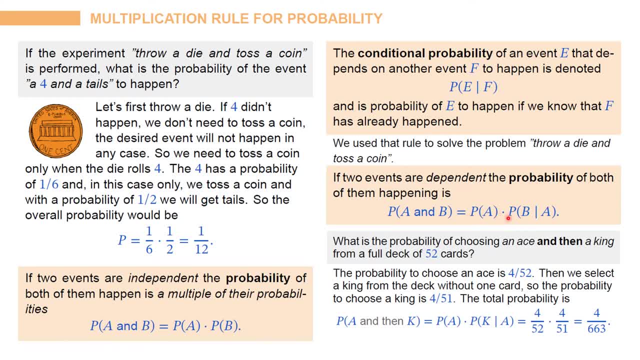 P of A times P of B, the conditional probability of B. So let's look at an example: What is the probability of choosing an ace and then a king from a full deck of 52 cards? Okay, so first, why is this a conditional probability problem? It's because the probability 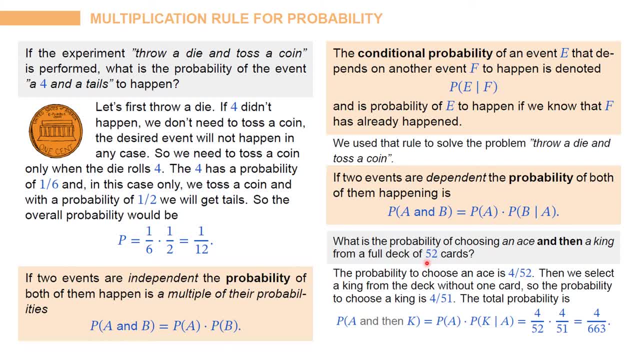 of drawing the second card depends on what happened when you drew the first card. There are no longer 52 cards in the deck, There are 51, and in this case we know that the king was not drawn because we drew an ace. So the probability to choose an ace- 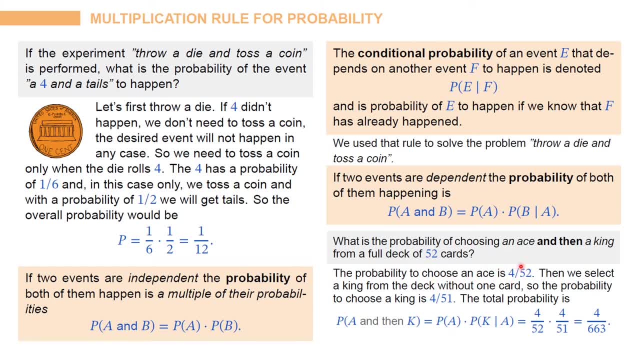 first is 4 out of 52.. Four aces out of the 52 cards. Then we select a king from the deck without one card and we know this card had to be an ace. so the probability to choose a king is 4 in 51.. 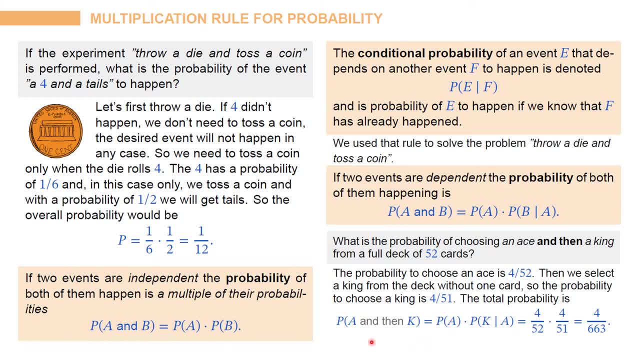 The total probability is P of an ace and then a king equals P of drawing an ace times the probability of drawing an ace. So the probability of drawing a king after we have drawn an ace. So this is equal to 4 over 52 times 4 over 51, which is equal to 4 over 663. 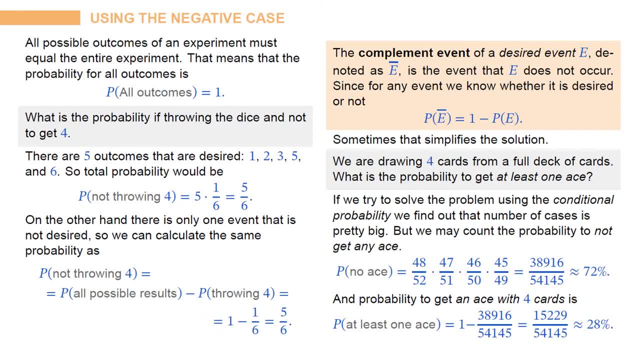 Now it turns out sometimes it's easier to calculate the probability of something not happening than the probability of it happening, and so using that negative case is often very convenient. It's because all possible outcomes of an experiment must equal the entire experiment. That means that the probability for all outcomes is equal to 1. So there's a 100% chance that one 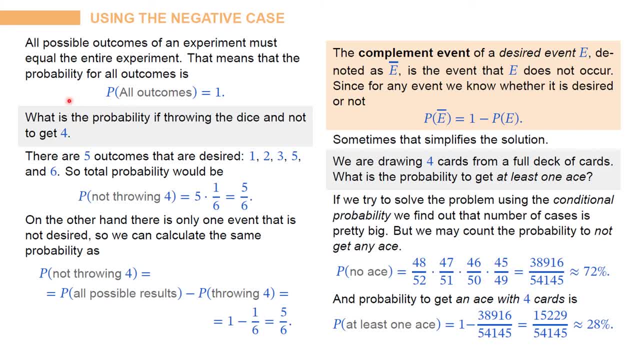 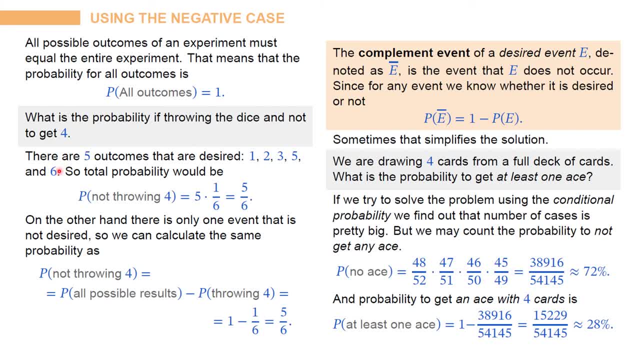 We have omitted the four, So the probability would be five times one sixth, because there's an equal probability: 1 sixth of either of those five numbers, So it's 5 sixths. On the other hand, there is only one event that's not desired, so we could have also calculated this. 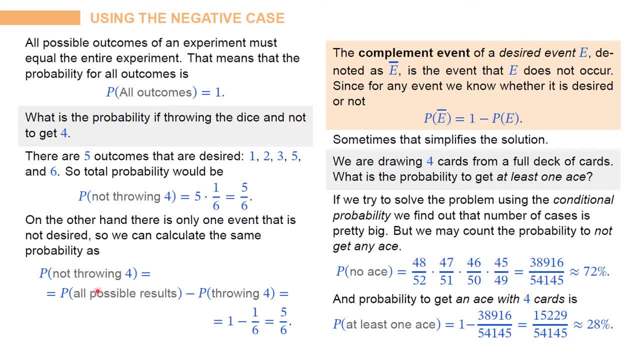 by saying: the probability of not throwing a four is equal to the probability of all possible results, which is 1,, minus the probability of throwing a 4, which is 1, 6.. So we also get 1 minus 1, 6,, which equals 5, 6.. The complement event of a desired event, E, is denoted by E. 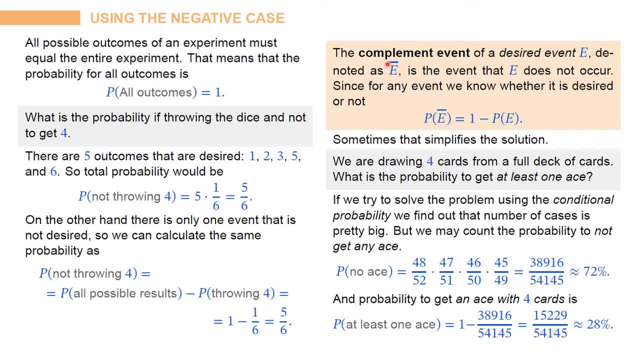 with a bar over it, It is the event that does not occur. So, in other words, the complement to rolling a 4 is rolling a 1, 2, 3, 5 or 6.. Since, for any event, we know that either the desired event or the undesired event has to happen, the complement probability. 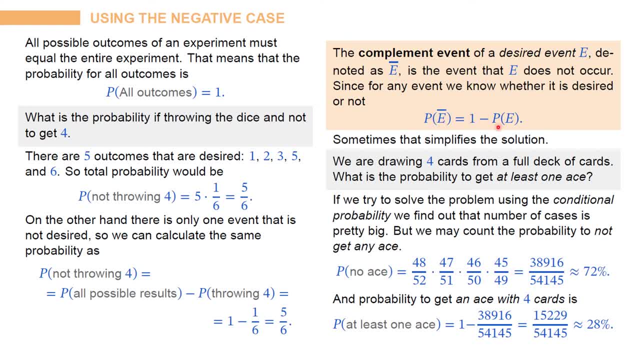 is equal to 1 minus the probability of the event. Now, this term complement is probably familiar to you from right angle. If you have two angles, they sum to 90. Suppose you have angle A, its complement angle B is 90 minus angle A. There the angles have to sum to 90 degrees. Here the probabilities. 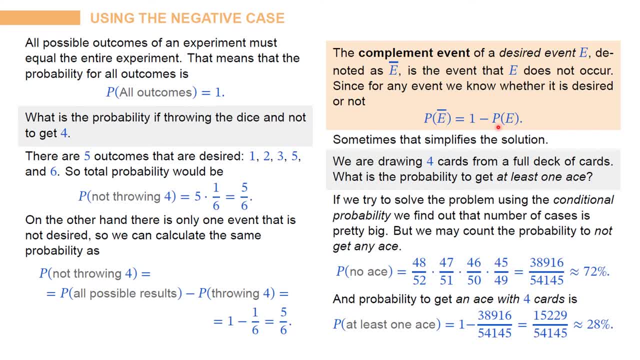 have to sum to 1, and the complement of an event is 1 minus the probability of the event. As I've mentioned, sometimes using this complement really helps simplify a solution. We are drawing four cards from a full deck of cards. What is the probability that we get at least one ace? Well, one way. 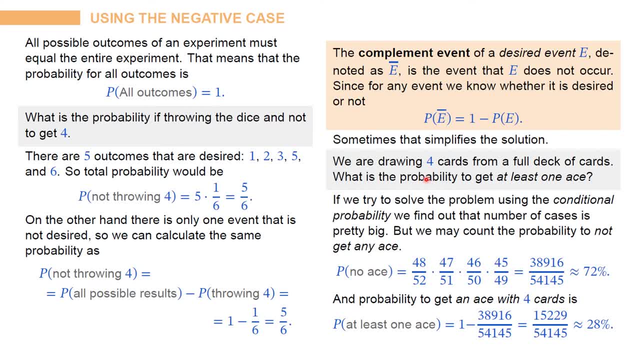 to solve this would be the probability of getting one ace plus the probability of getting two aces, plus the probability of getting three aces, plus the probability of getting four aces and then adding all of those up. But that's actually a little bit hard to do. 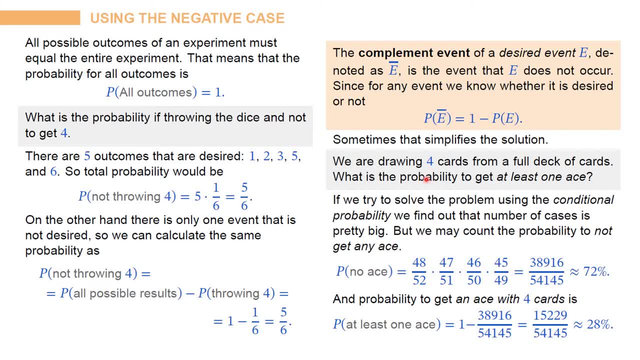 It is much easier to figure out the probability that we do not get an ace and then subtract that from one, And by the rules of this negative case we know that we have then solved for the probabilities of getting at least one ace, So the probability of not getting an. 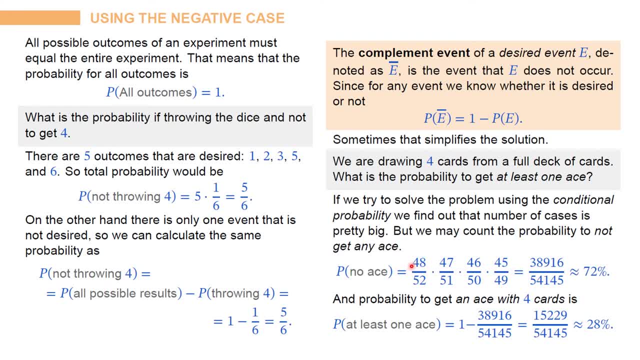 ace is: you don't draw an ace on the first one. There are 48 aces in the first one and there are 48 non-aces out of 52 cards. Then we don't draw an ace on the second one Now. 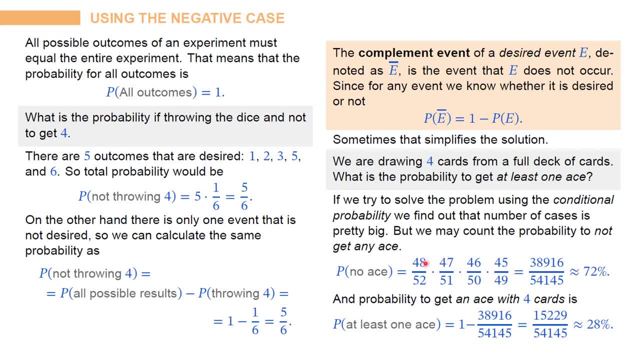 since you didn't draw an ace on the first event, there are now 47 non-aces out of the 51 cards. Then we haven't drawn an ace on the first two, so not drawing an ace on the third card is a 46 out of 50 probability. And finally, since we haven't drawn an ace, 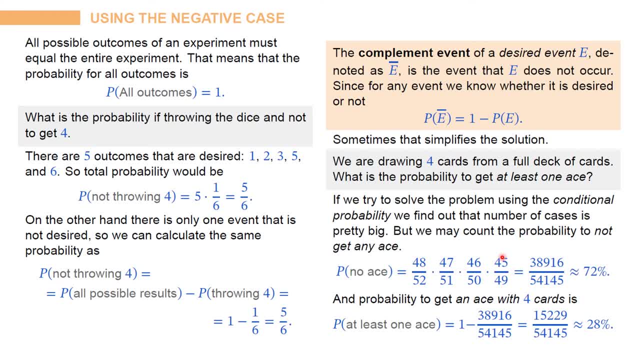 yet the probability of not drawing an ace on the fourth and final card is 45 out of 49.. We use a calculator and we get this is around 72 percent. So the probability that we get at least one ace with four cards is one, minus the probability that 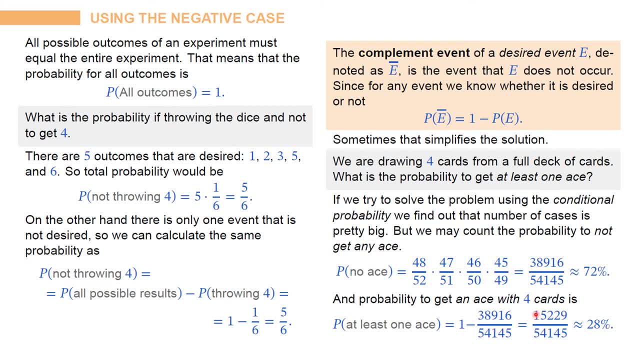 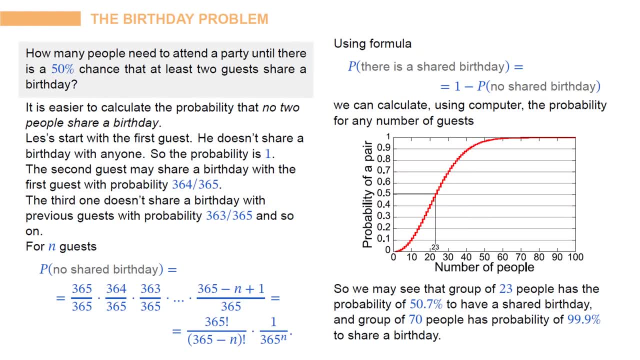 we didn't get an ace which, in fractional form, is exactly this and is approximately equal to 28 percent. A cool and very famous example where it turns out using this negative probability is very handy is the birthday problem. It is stated usually this way: How many people need? 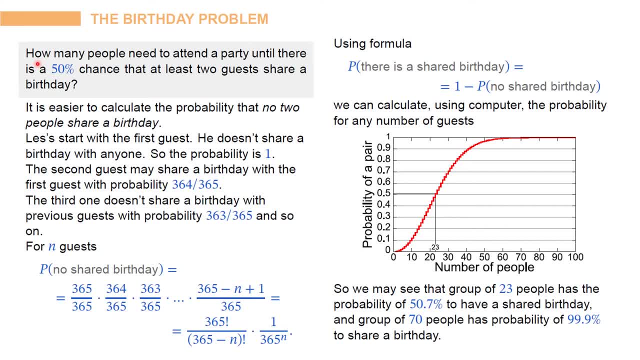 to attend a party until there is a 50 percent chance that at least two guests share a birthday. Okay, as I mentioned, it's easier to calculate the probability that no two people share a birthday. Let's another typo: start with the first guest. He doesn't share a birthday with anyone, so the probability is one If there's. 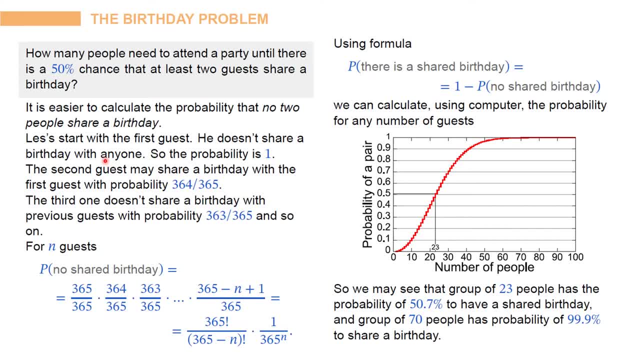 only one guest. there's a 100 percent chance that no two guests share a birthday. The second guest arrives, Well, he has a birthday, and there is now a one in 365 chance that their two birthdays are the same same. if we ignore leap years, which, to the accuracy of this problem, is fine. So the probability that 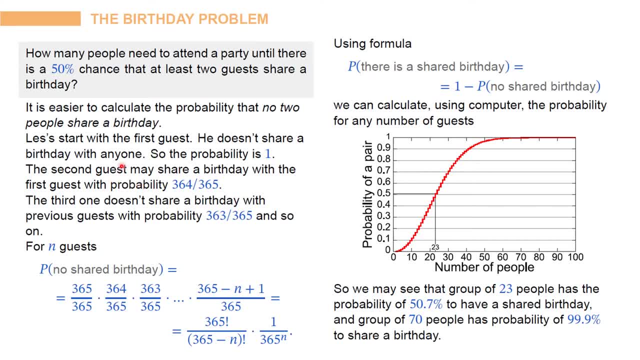 you do not share a birthday, so sorry for that. the probability that you do not share a birthday is 364 over 365.. Okay, so the probability if the first two guests don't share a birthday, that the third guest doesn't share a birthday is 363 over 365, and so on. So for n guests, the probability 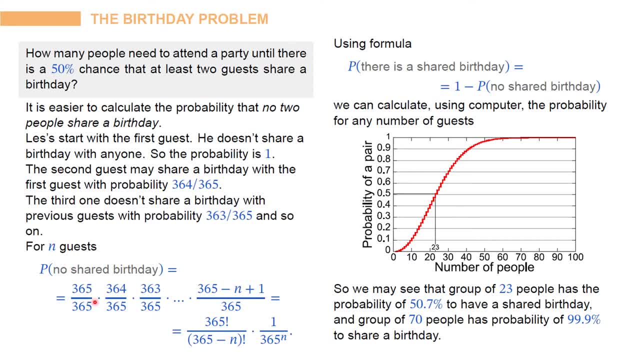 that there is no shared birthday is 1 times 364 over 365 times 363 over 365.. You see the pattern. for the nth guest, we'd go until 365 minus n, plus 1 over 365.. And when we multiply: 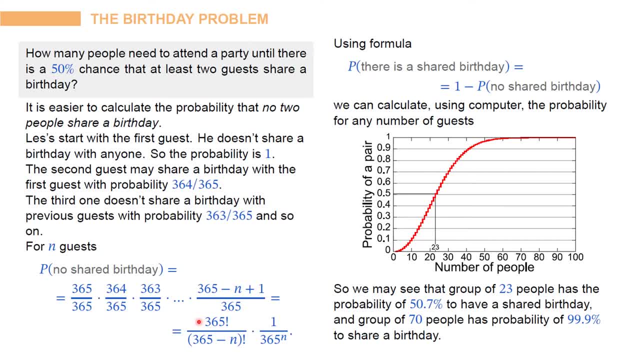 all of these together, we get 365 factorial over 365 minus n factorial. right, That's how we ended up with the 365 minus n plus 1 over 365. Multiplying times, you know one greater the whole series. then we have to multiply it by 1 over 365 to the nth power. So this might seem. like a little bit of a problem, but it's not. So we're going to multiply it by 1 over 365 to the nth power. So we're going to multiply it by 1 over 365 to the nth power. So we're going to. 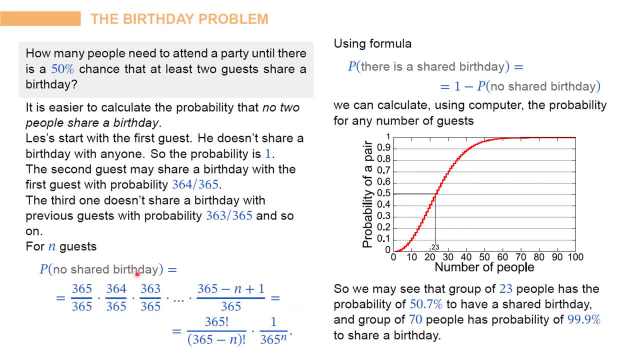 an intimidating formula, but think about how we got it. We just started with the first guest and the second guest didn't share a birthday, and then we multiply that by the third guest not sharing a birthday, and so on. So now to figure out the probability that there is a. 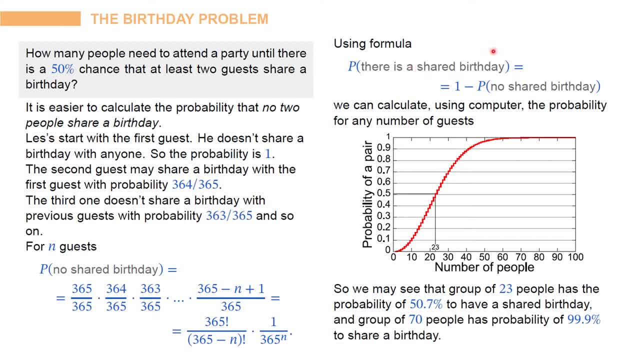 shared birthday. we simply subtract the probability that there isn't a shared birthday from 1, and this is way too complicated to calculate by hand. So you plug this, this formula, into a computer and you can get a graph of the probability of sharing a pair. 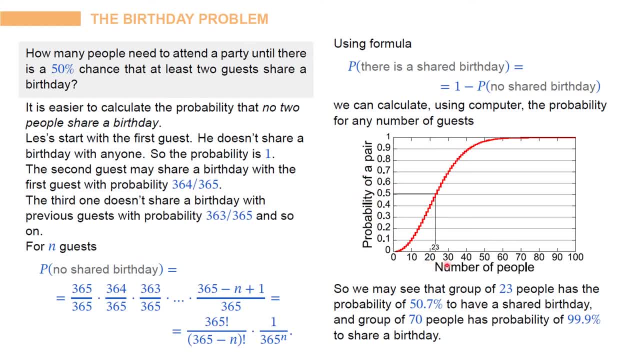 of birthdays, at least one pair of birthdays divided, plotted versus the number of people, and you see that when 23 people are at the party, we finally crossed the 50% threshold and it is now 50.7% chance that there is at least one shared birthday, And this you know. 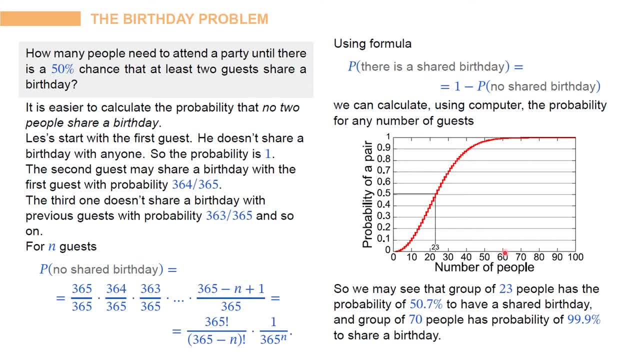 very quickly approaches one. By the time you have 70 people, there's a problem. there's a 99.9% probability that there's at least a shared birthday And if you got, you know, 300 people, it would be 99.many. 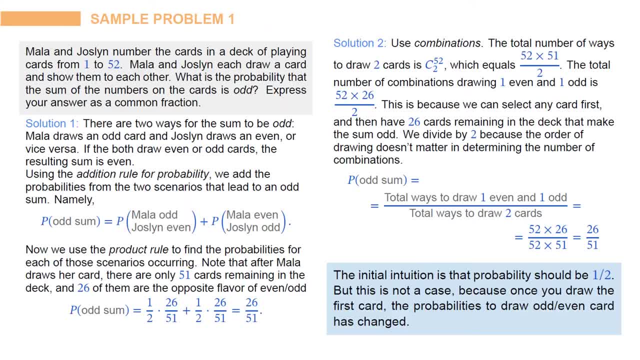 nines after that. Now let's do a couple sample problems where we get to apply multiple counting techniques to help us come up with the probability. So we've already learned combinatorics. That's going to be very useful in calculating the number of outcomes, and we need to know the desired outcomes versus the total outcomes to 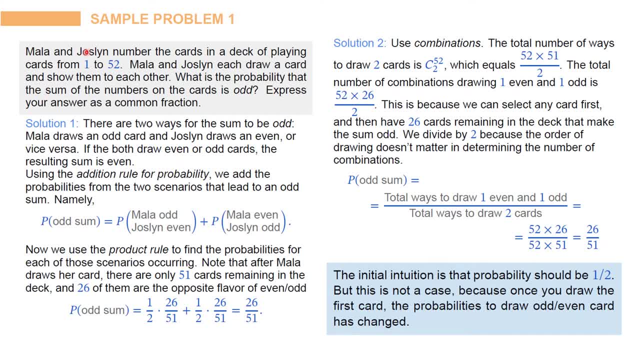 calculate probability. So Mala and Joslyn number the cards in a deck of playing cards from 1 to 52. So ignore what's normally on the cards. We have 52 pieces of paper numbered 1 to 52. Mala and 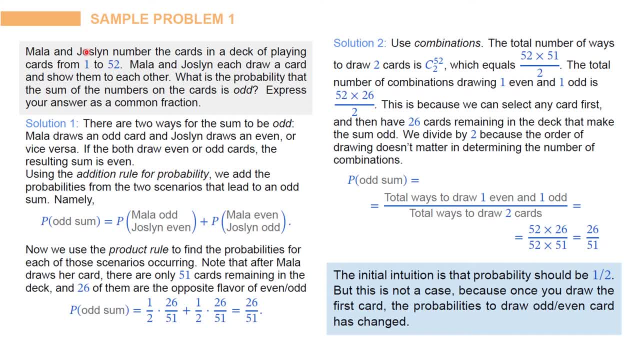 Joslyn each draw cards from 1 to 52.. So we have 52 pieces of paper numbered 1 to 52.. Mala draws a card and shows them to each other. What is the probability that the sum of the numbers on the cards is odd? Express your answer as a common fraction. So there are two ways to do it. 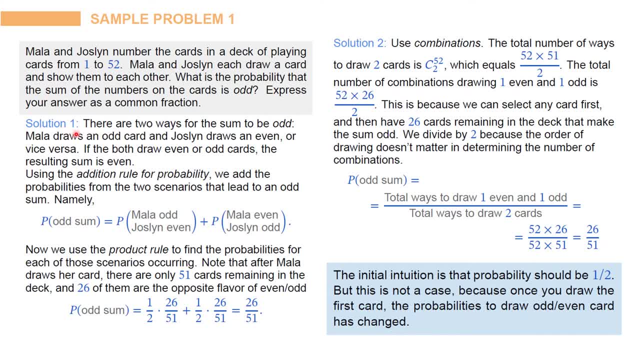 Let's look at solution one. There are two ways for the sum to be odd: Mala draws an odd card and then Joslyn draws an even, or vice versa, If both of them draw even cards or both draw odd cards. 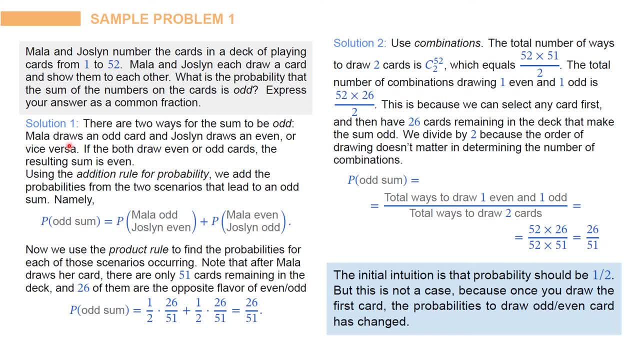 the resulting sum is even Using the addition rule for probability, we add the probabilities from the two scenarios that lead to an odd sum, Namely P odd equals P Mala odd Joslyn even plus P Mala even Joslyn odd. That's okay to do. 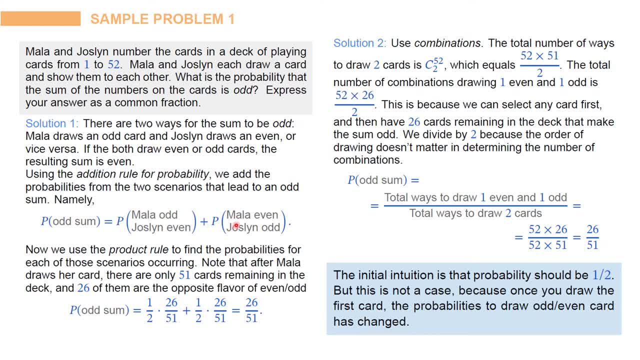 Because these two events cannot both happen. So we have two independent events, no overlap. We add the probabilities of the two events. What is the probability of this event happening? We use the product rule to find the probabilities for each of these scenarios. 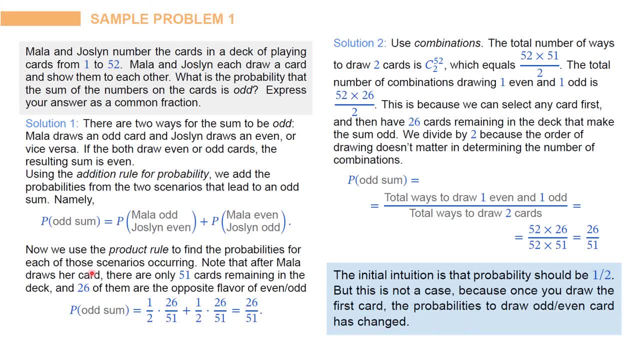 So note that after Mala draws her card, there are only 51 cards remaining in the deck, and 26 of them are the opposite flavor. The probability of an odd sum is two things. One is that each of these scenarios are equal. two of them are equal. 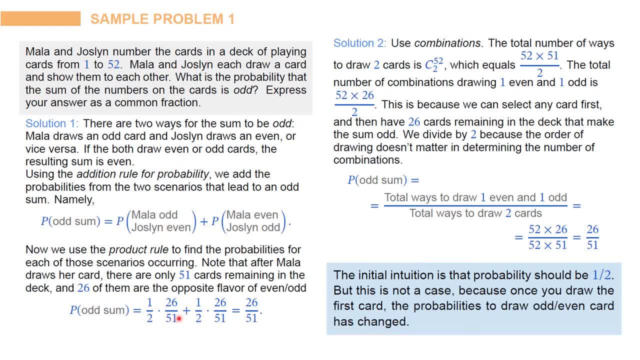 So the probability of an odd sum is one half times 26 over 51.. That was the odd even scenario Plus one half times 26 over 51. That was the even odd scenario. That's equal to 26 over 51.. 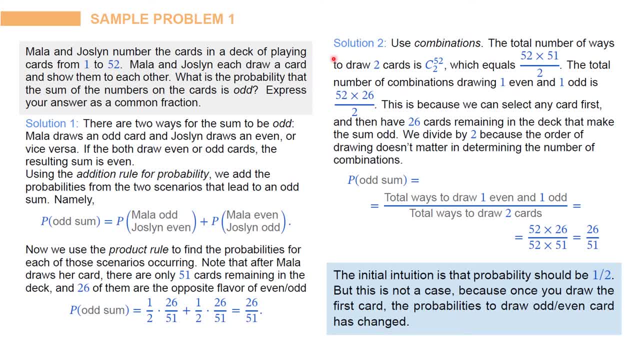 So here's solution two. We could have used combinations. total number of ways to draw two cards from a deck of 52 is 52. choose two. That's using this combination notation, Choose two out of 52, and remember that's equal to 52 times 51 divided by. 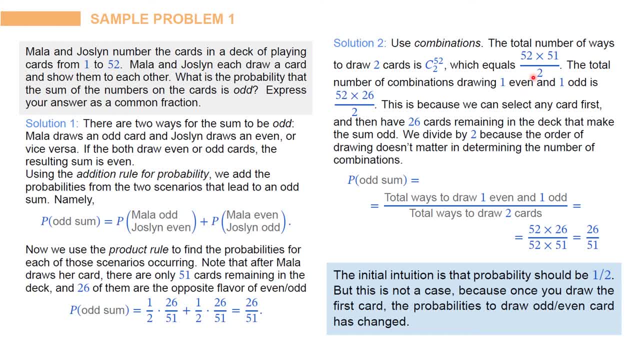 2 factorial. right, because it was 52 factorial divided by 52 minus 2 factorial, so that was 50 factorial. so that got rid of all the factors less than 51, and then this is the 2 factorial and the bottom is 2.. The total number of combinations drawing one even and one odd. 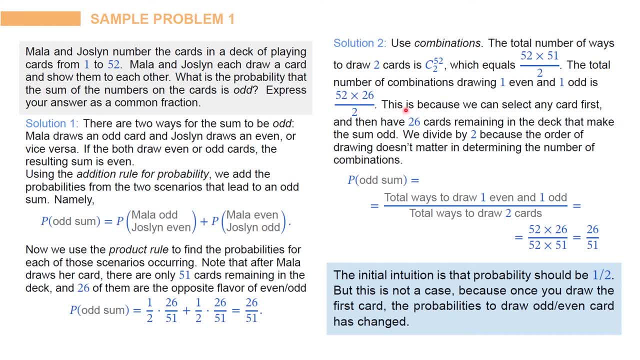 is 52 times 26 divided by 2.. This is because we can select any card first and then have 26 cards remaining in the deck that make the sum odd. We divide by 2 because the order of drawing doesn't matter in determining the number of combinations, So the probability of an odd sum are the total. 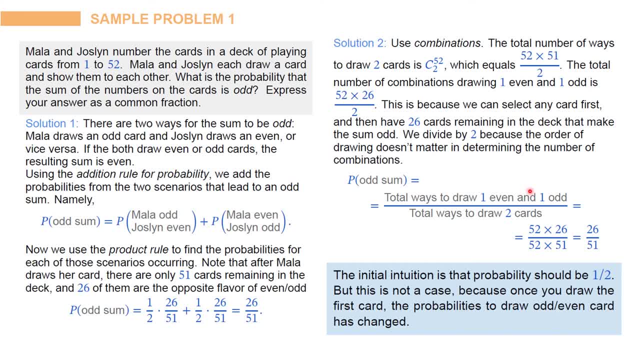 number of ways to draw one even and one odd divided by the total number of ways to draw two cards. so this is 52 times 26 divided by 52 times 51, and fortunately the second solution agrees with the first solution, as it has to, if our counting was correct. now your initial into. 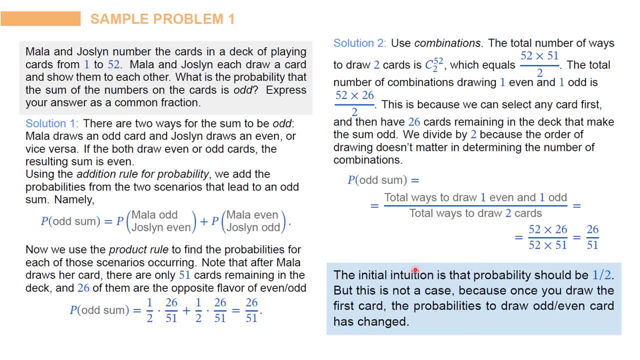 intuition was probably that the probability should have been one half. this is not the case, because once you draw the first card, you have broken the symmetry of odd. even in drawing the second card, it's always going to be more likely that you draw the opposite flavor than what you originally. 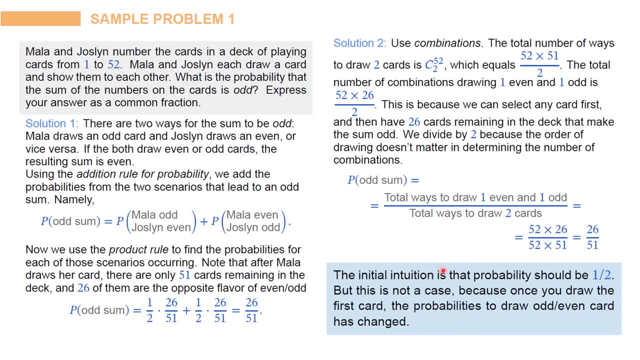 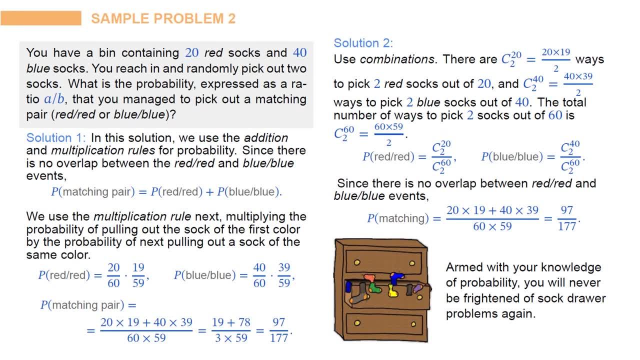 drew, and that's why the probability of getting an odd sum is a little bit over one half. okay, sample two: the infamous sock drawer kind of question sometimes. Sometimes it's marbles of different colors, Sometimes it's socks of different colors, but you get the idea. 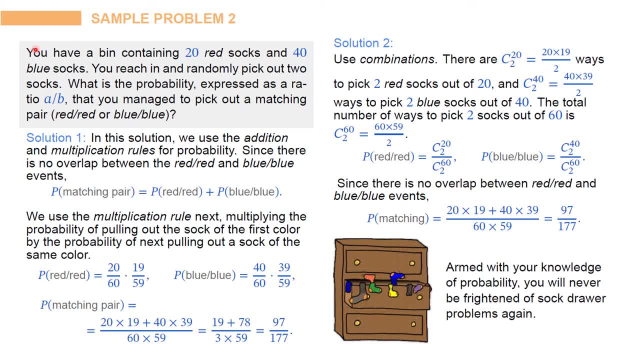 You'll see a lot of questions like this. You have a bin containing 20 red socks and 40 blue socks. You reach in and randomly pick out two socks. What is the probability, expressed as a ratio A over B, that you managed to pick out a matching? 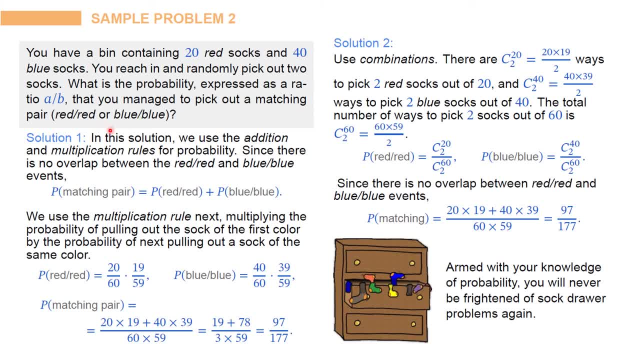 pair, red-red or blue-blue. Again, we could count in two ways. Let's look at solution one. In this solution we use the addition and multiplication rules for probability. Since there is no overlap between the red-red and blue-blue events, the probability of a 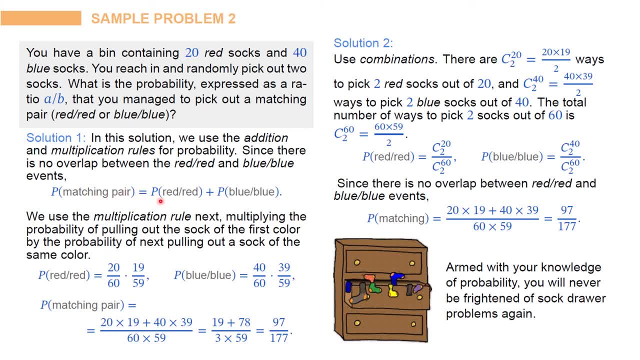 matching pair is simply the addition: the sum of P red-red plus P blue-blue. Next we use the multiplication rule. multiplying the probability of pulling out a sock of the first color, Multiply the probability of next pulling out a sock of the same color. 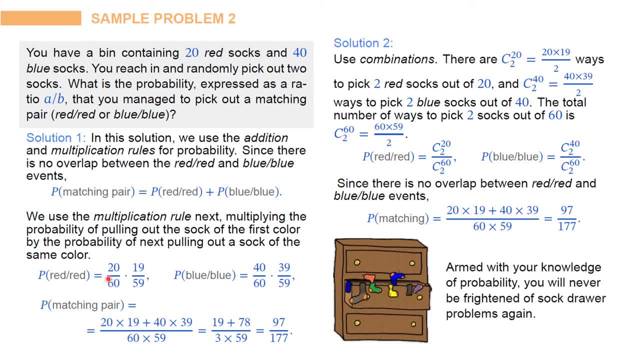 P red-red is equal to the 20 over 60 chance of pulling out a red sock times the conditional probability- 19 over 59- of pulling out a red sock, assuming you've pulled out a red sock. second, if you already pulled out a red sock, because there are 59 socks left in the drawer, 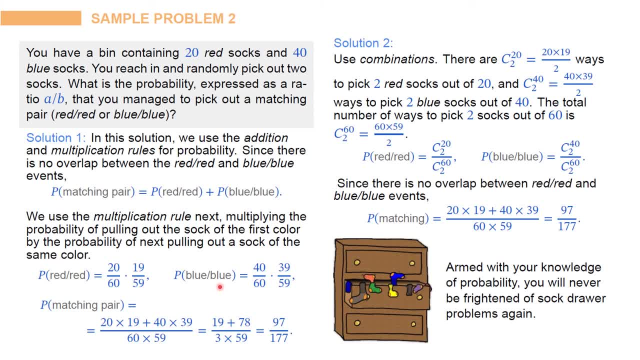 and only 19 of them are red. Similarly, P blue-blue is 40 over 60 times 39 over 59,, as we started with 40 red socks. So the probability of a matching pair is 20 times 19 plus 40 times 39 divided by their. 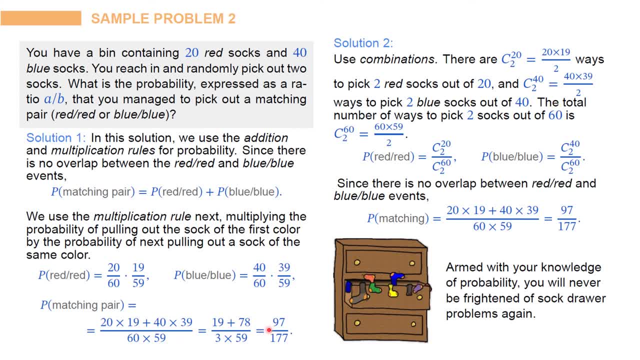 common denominator 60 times 59, and this simplifies to 97 over 177.. Now let's solve the problem another way. Use combinations, Again, Remembering we have 20, choose 2, so that simplifies using the formula for combinations. 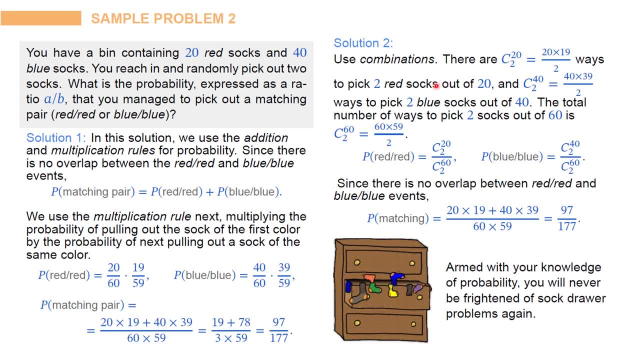 to 20 times 19 over 2 ways to pick 2 socks out of 20.. Okay, So that's how many ways we could pick a pair of red socks, And then how many ways could we pick a pair? I mean, I'm sorry, that was how many ways. 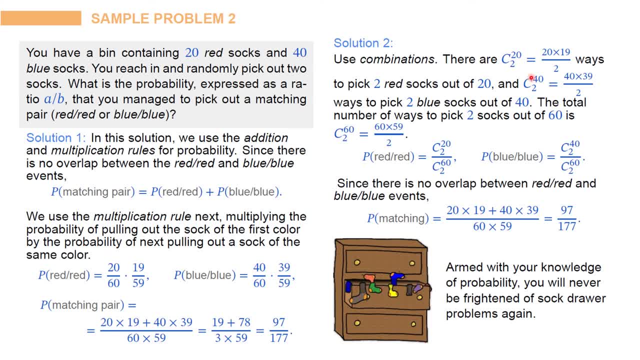 how many ways were there to pick a pair of red socks? Well, there are 40 blue socks. you want a pair? so that's 40, choose 2, using our formula, that's 40 times 39 divided by 2.. 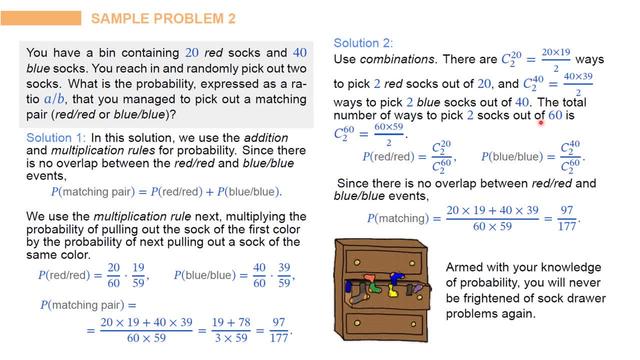 What is the total number of ways to pick 2 socks out of 60? That's 60 choose 2, so 60 times 59 over 2.. Okay, So P red-red is 2 choose 20 divided by 2.. 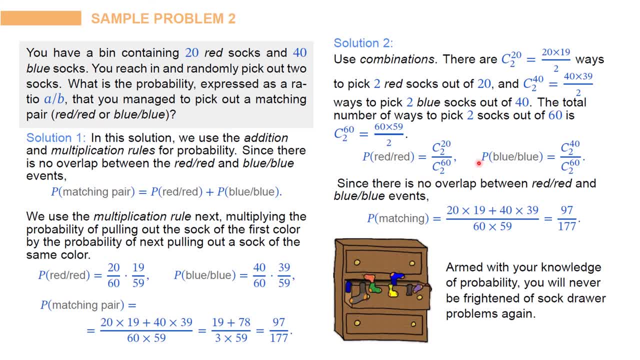 Okay So P red-red is 2, choose 20 divided by 2.. Okay So P blue-blue is 2 chews 60,. P blue-blue is 40. choose 2 divided by 60, choose 2.. There's no overlap. 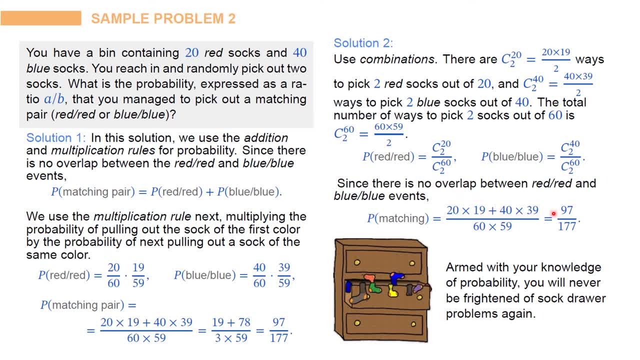 So again we add them and we get the same answer: 97 over 177.. So now that you know these rules for probability, you will be never frightened of sock drawer problems again, except like if they're throwing argyle socks. Okay, 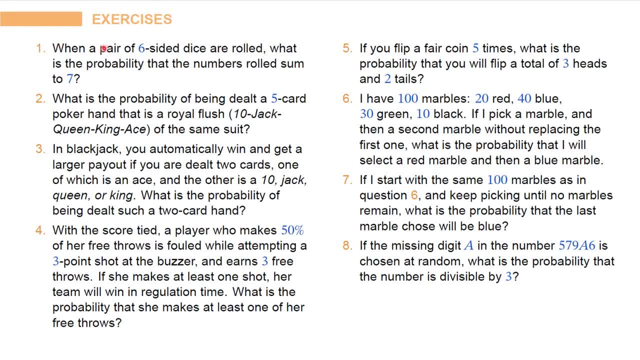 Okay. So that to me that was all Okay. what are the exercises for this week? Number one: when a pair of six-sided dice are rolled, what is the probability that the numbers rolled sum to seven? By the way, seven is the most likely. 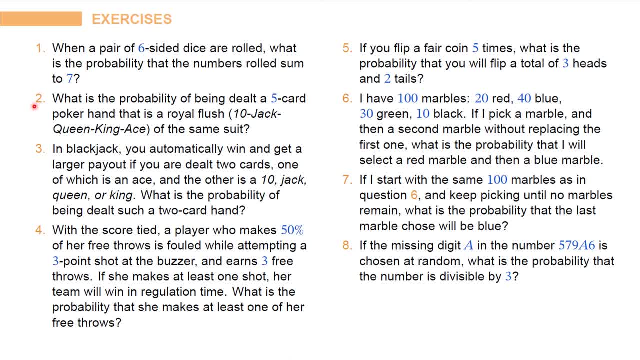 outcome of rolling a pair of dice? Number two: what is the probability of being dealt a five-card poker hand, that is, a royal flush- ten jack, queen, king, ace- of the same suit? So of course, there are four possible suits with royal flushes. So what is the probability of getting a royal? 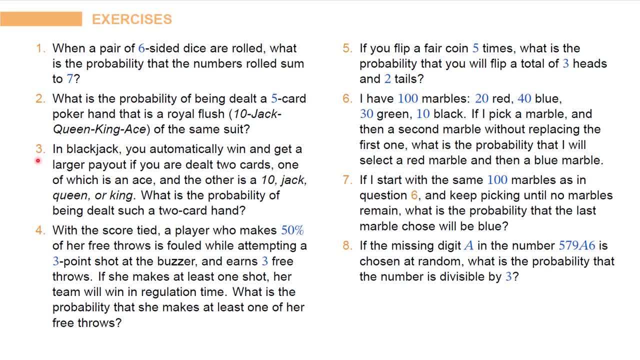 flush in any of those suits. Number three: in blackjack, you automatically win and get a larger payout if you are dealt two cards, one of which is an ace and the other is a ten jack, queen or king. What is the probability of being dealt such a two-card hand and the order of which? 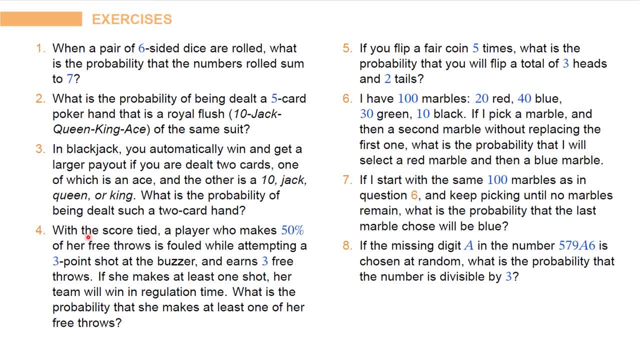 cards Number four. with the score tied, a player who makes 50% of her free throws is fouled while attempting a three-point shot at the buzzer and earns three free throws. If she makes at least one shot, her team will win in regulation time. What is the probability that she makes at least? 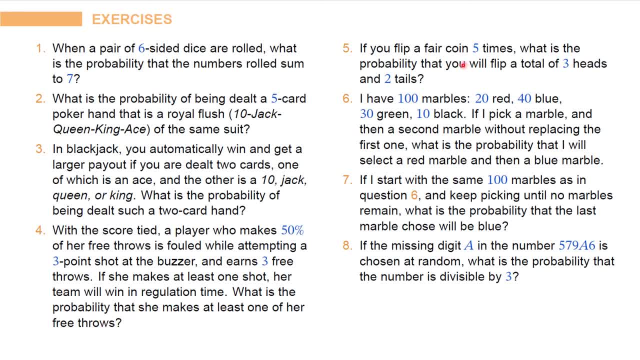 one of her free throws. Number five: if you've got a three-point shot at the buzzer, if you flip a fair coin five times, so that means it's a 50% chance of heads and 50% chance tails on each flip. what is the probability that you will flip a total of three heads? 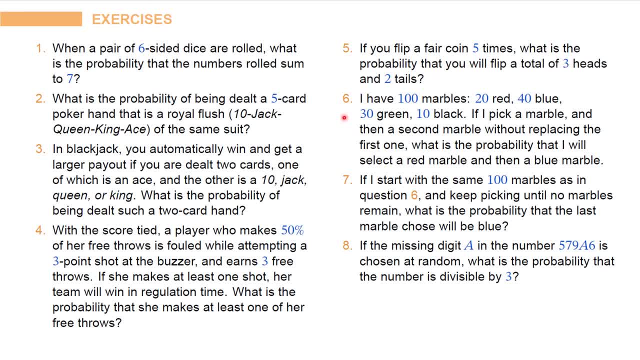 and two tails. Number six: I have 100 marbles: 20 red, 40 blue, 30 green, 10 black. If I pick a marble and then a second marble without replacing the first one, what is the probability that I will select a red marble and then a blue marble in that order? Number seven: if I start 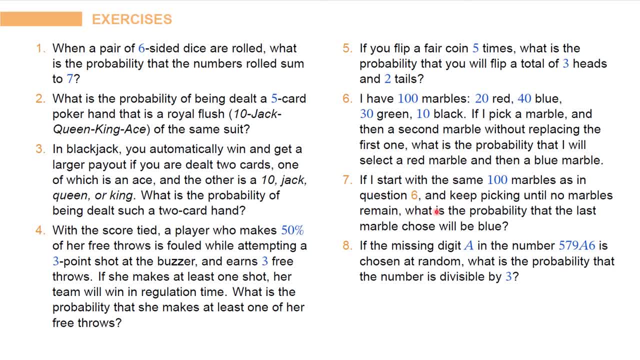 with the same 100 marbles as in question six and keep picking until no marbles remain, what is the probability that the last marble chosen will be blue And eight. if the missing digit A in the number 579A6 is chosen, what is the probability that the last marble chosen will be blue? 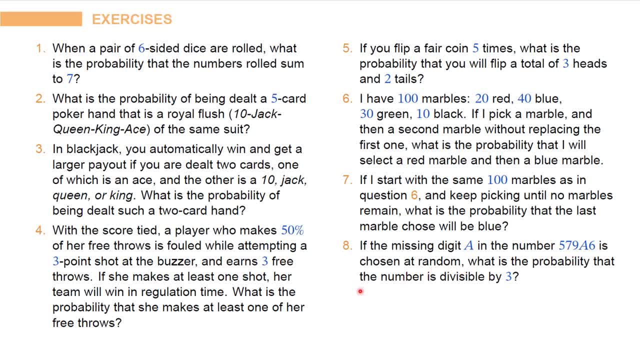 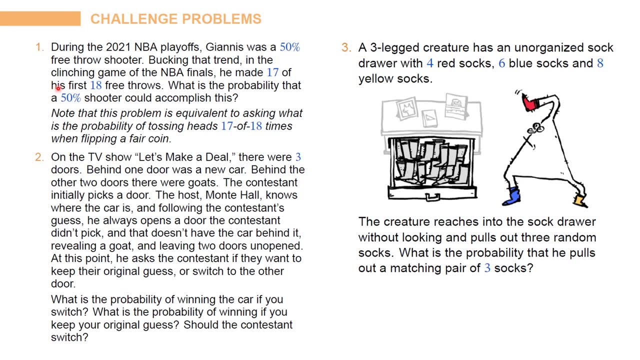 Number seven. if the last marble chosen is chosen at random, what is the probability that the number is divisible by three? So here we're trying to be a little cumulative, going back to our divisibility rule lesson, so you don't forget your divisibility rules. And finally the challenge. 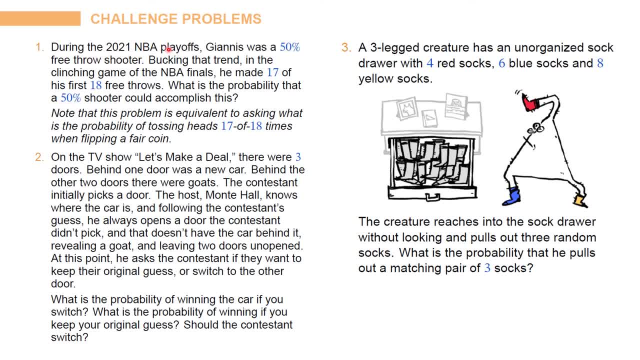 problems for this week. During the 2021 NBA playoffs, Giannis was a 50% free throw shooter. Bucking that trend: Get the job done. He played for the Bucs, so I used the phrase. bucking that trend means going against that trend. 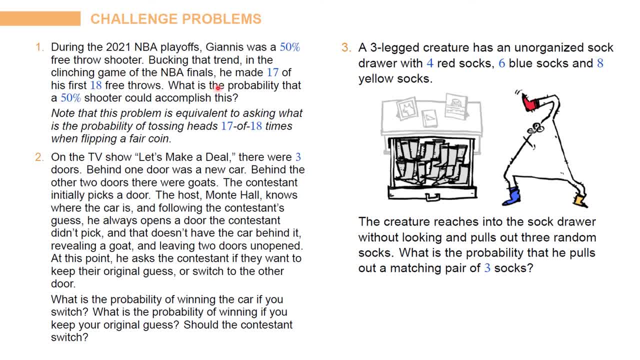 Bucking that trend. in the clinching game of the NBA finals, he made 17 of his first 18 free throws. What is the probability that a 50% shooter could accomplish this? Note that this problem is equivalent to asking what is the probability of tossing heads 17 of 18 times when flipping a fair. 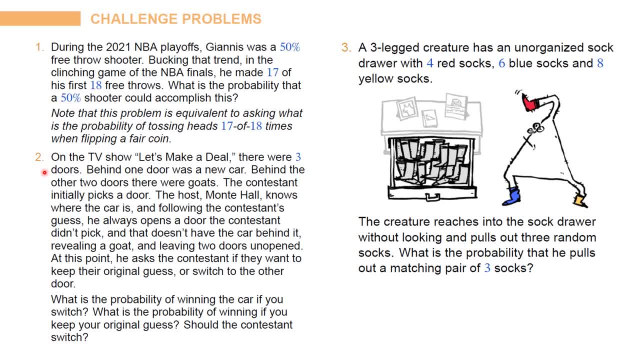 coin. Number two is a very famous probability question called the Monte Hall problem. On the TV show Let's Make a Deal, there were three doors. Behind one door was a new car. Behind the other two doors there were goats. The contestant initially picks a door. The host, Monte Hall, knows where the car is. 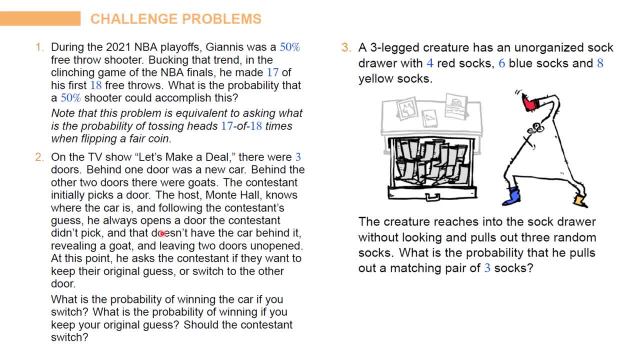 and, following the contestants, guessed. he always opens a door the contestant didn't pick. and that doesn't have a car behind it, Revealing the contestant. the door didn't win: 20 points, revealing a goat and then leaving two doors unopened. At this point, he asked the contestants. 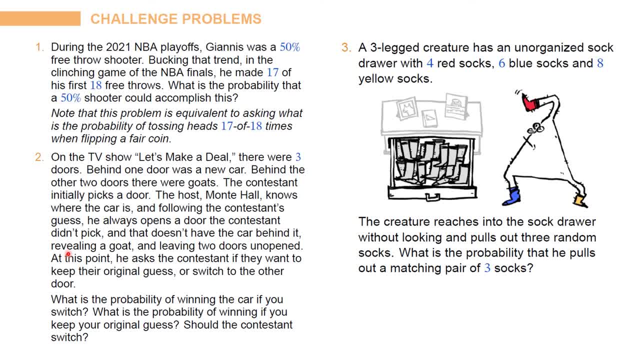 if they want to keep their original guest or switch to the other door. What is the probability of winning the car if you switch? What is the probability of winning the car if you keep your original guest, Should the contestant switch? Finally, number three, A three-legged creature has. 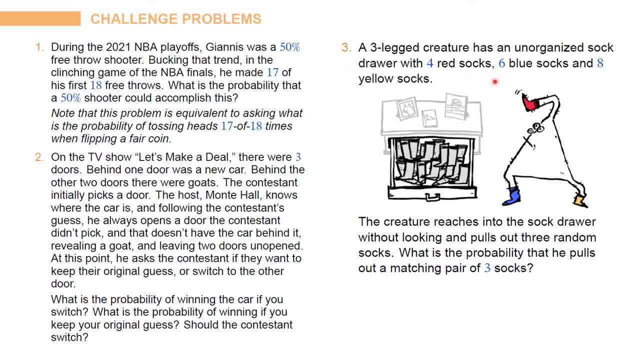 an unorganized sock drawer with four red socks, six blue socks and eight yellow socks, And it's dark so you can't see what color they are. The creature reaches into the sock drawer without looking and pulls out three random socks. What is the probability that he pulls out a matching pair of three socks? Okay, that's it. for this week. See you guys in class. Thank you for watching.